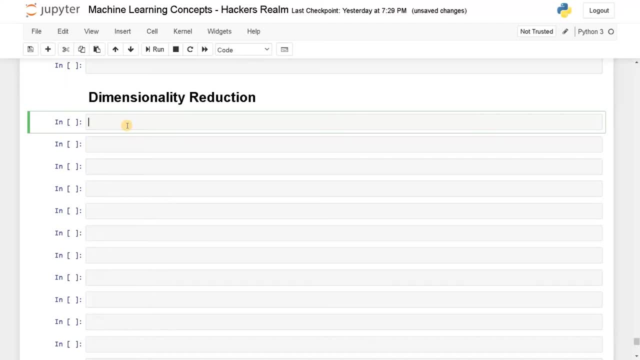 dive into the project now. First I will import the data. So from kerasdatasets import MNIST. So this is the dataset, Let's load it So it will be splitted into like train and test. So I am going to get only train data. 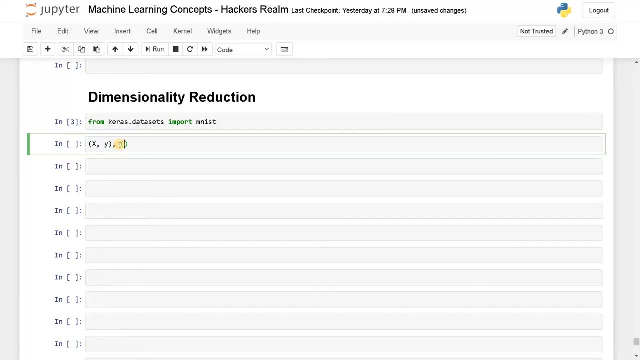 So that is enough for us. So this is one tuple and these two we don't need. Okay, this is underscore, It's like a temporary variable. Now here, mnistloaddata. Okay, this is the dataset And we will also check. 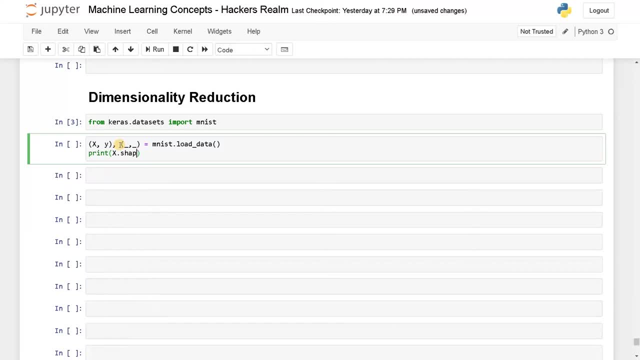 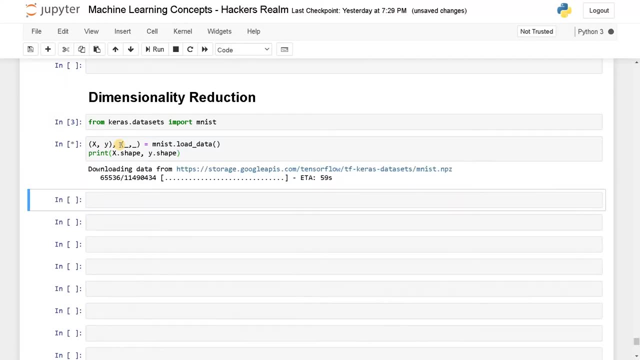 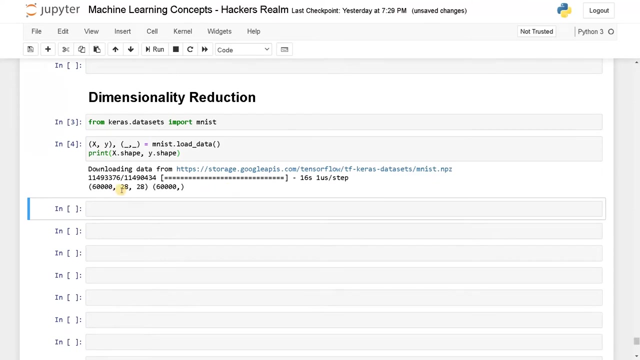 This is the shape, So print xshape and yshape and this. Now the data set has been downloaded. I think it's around like 114 MB, So it will be completed quickly. So this is the data set. We have around like 60,000 samples for the import. 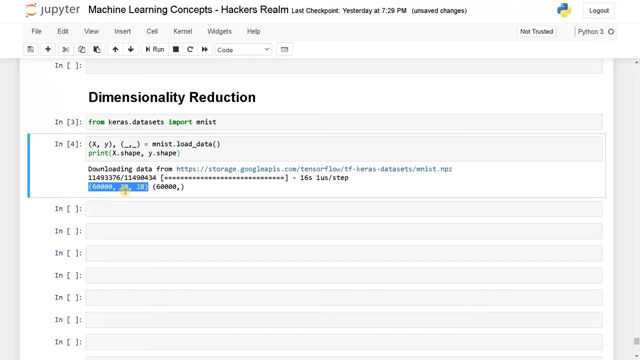 And the output. So this is the labels and this is the 28 cross 28 image pixel data. So we will just convert it into like a 1D array, like we are going to like flatten it. So I'm going to just flatten this data in order to get like a single dimensional array. 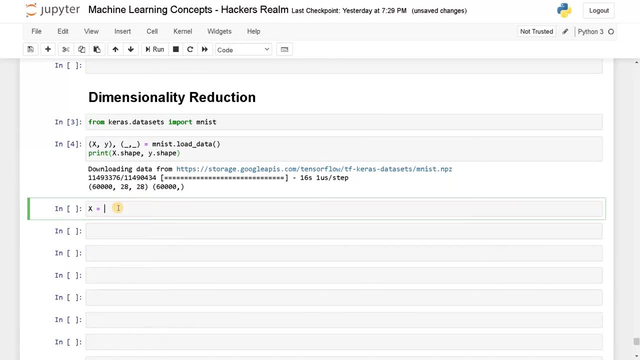 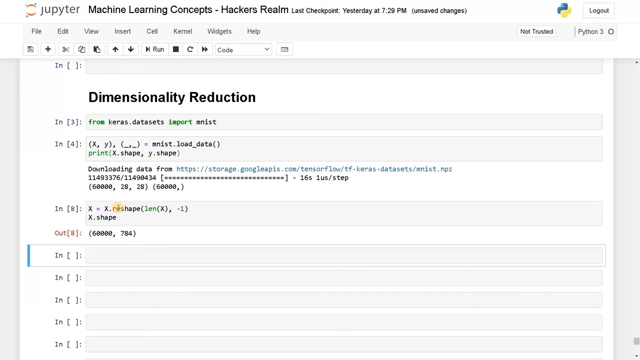 So for this I'm going to do: x equals x, dot reshape len of x. This is just the number of samples And remaining I'm just gonna flatten it And we will see the new shape here on this. So this is the new shape. 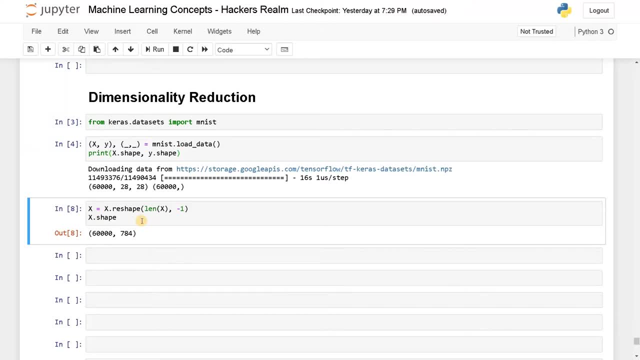 Now the data set has been loaded, Let's dive into the main functions. So we are going to implement all the feature reduction techniques First. I'm going to go with PCA, So before that I will import all the necessary modules for this. 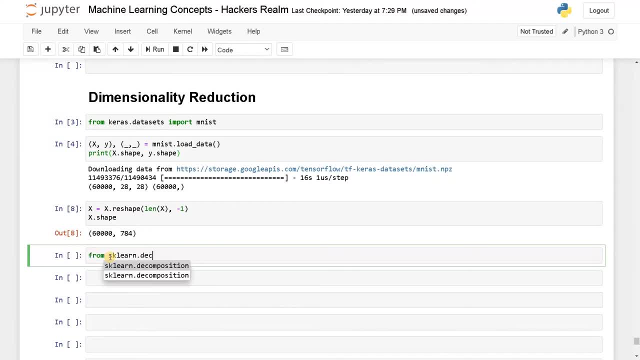 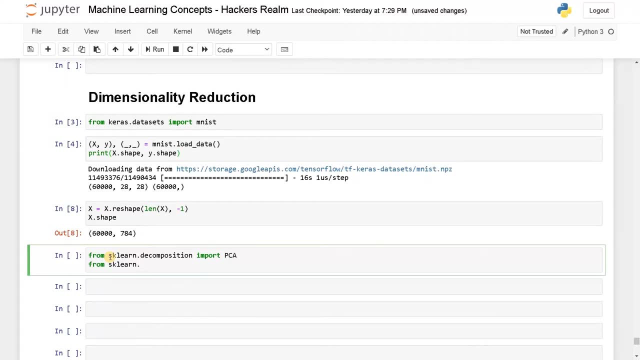 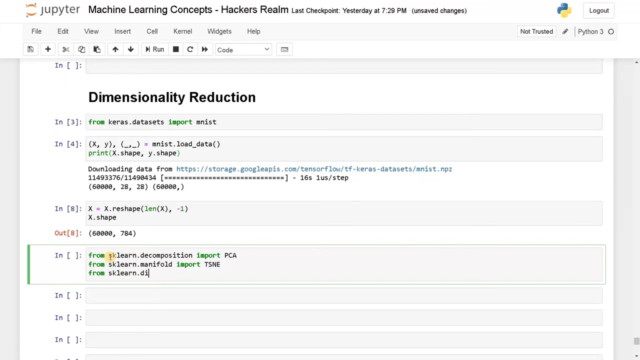 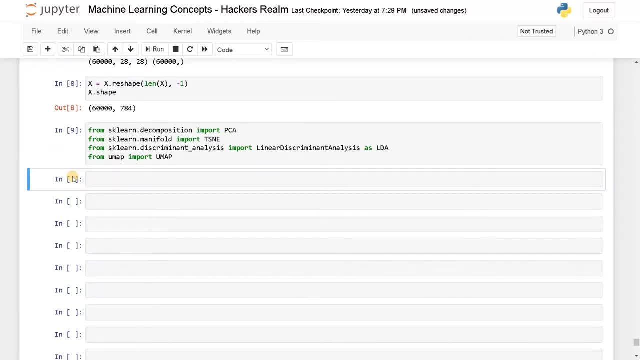 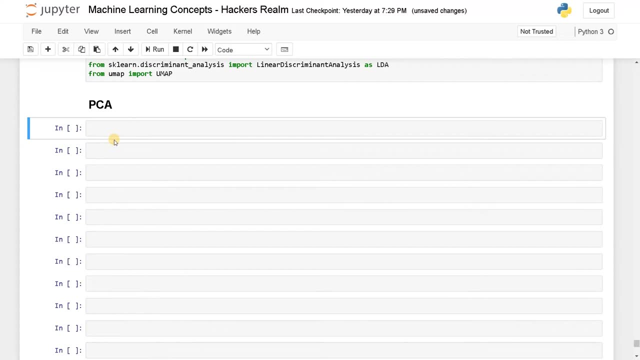 Okay, these are the modules we need. So first I'm gonna go with PCA, So we will just go one by one. So I will create a new variable called XPCA. xpca- it can be small itself, it's easy. now pca of n components: n components i'm gonna reduce. 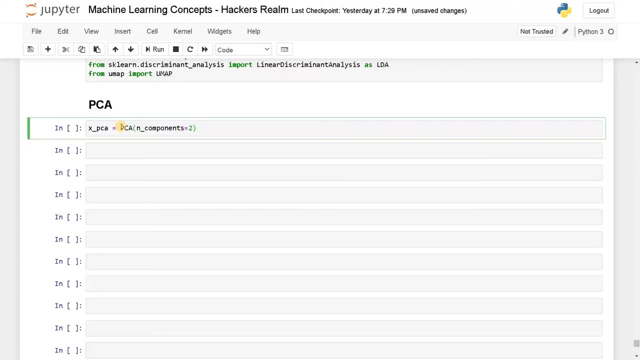 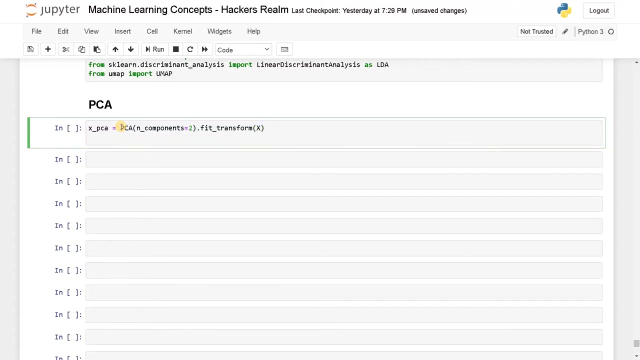 it to like two dimension in order to visualize it. so dot fit, transform, fit transform of x, comma y. sorry, we just need only the input. so this is like a unsupervised learning and after that we have to plot it. so i'll say: if plot dot figure, fix size. 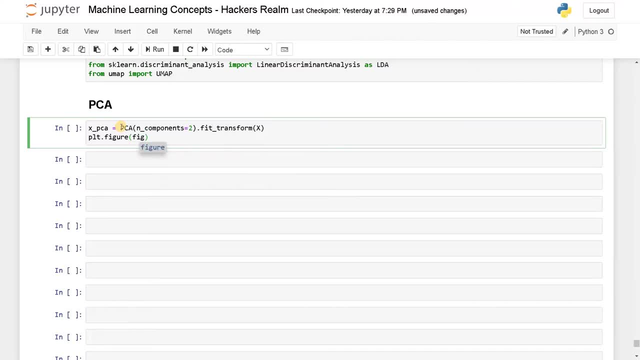 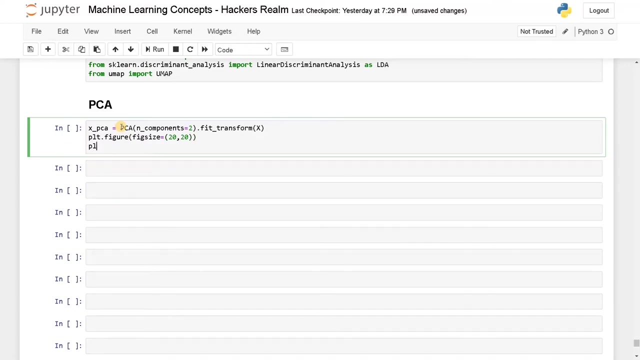 fig size equals. i can have like 20 comma 20, and after that we'll do the plotting. so plot dot scatter of x, pca of, we will get all the rows and we will get the zeroth column. so this is x axis. and similarly we will do the same for the y axis, so this will be one. and finally, 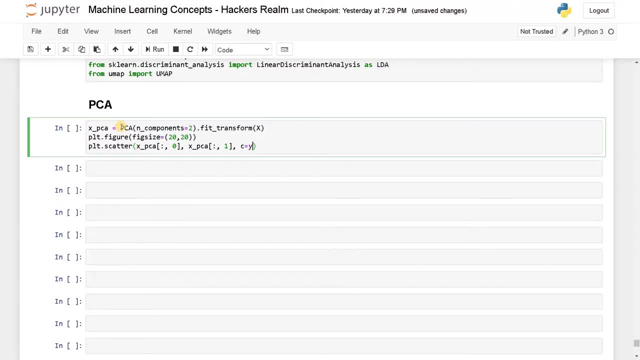 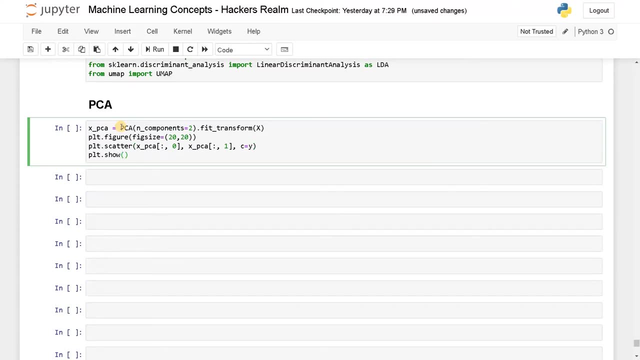 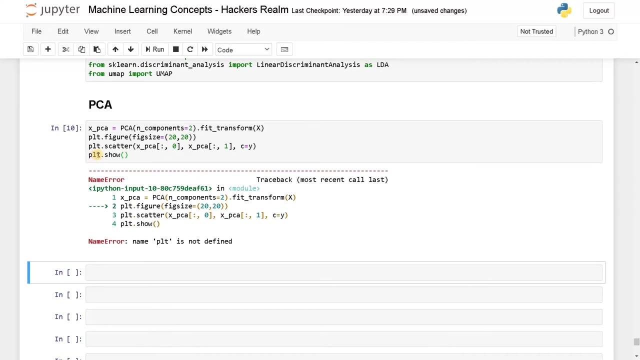 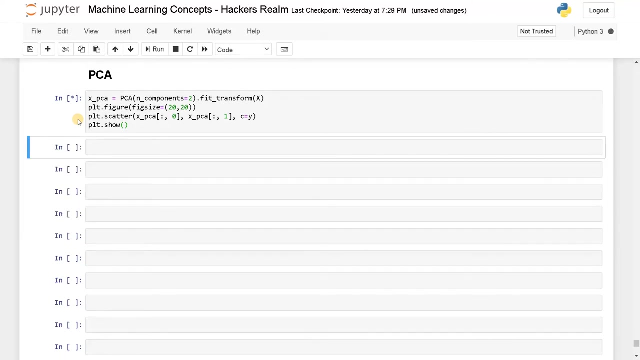 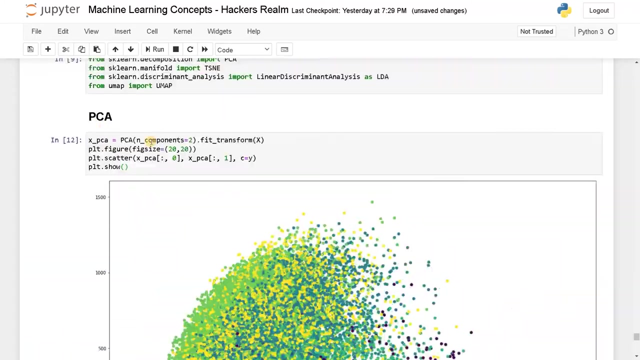 we have to have the colors. so that will be c equals y and i think that will be enough. let's say plot dot show, so this will just reduce the data. okay, plot is not yet imported. let's run this again now. we got a big data with all the different colors and we also need to have that data. 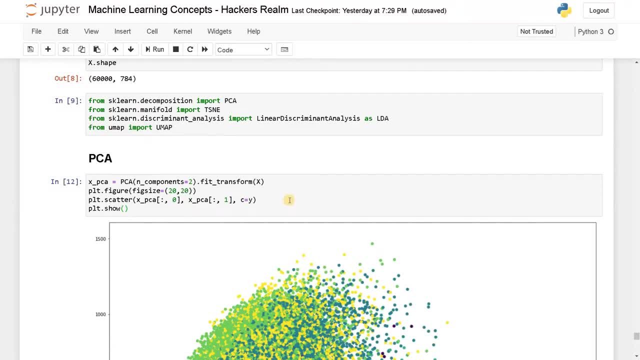 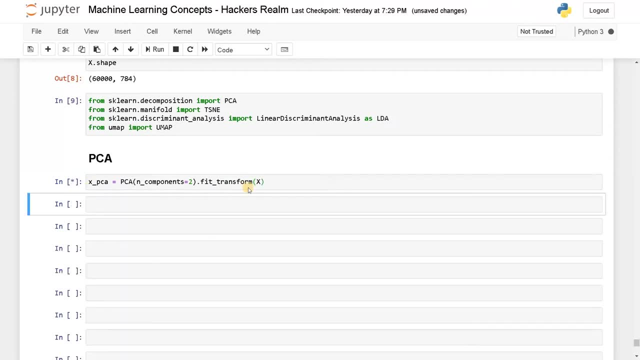 as Report in classroom and remember toЛarge data with lots of different colors and we that legend Let's see, So I'll just run it in a separate cell. We can also see the new shape, So dot shape see from 784, we have reduced it to like two dimension And 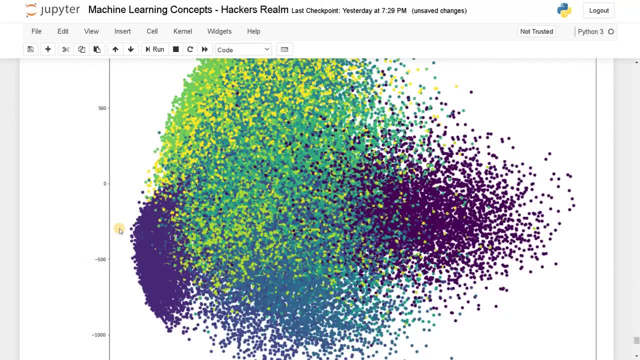 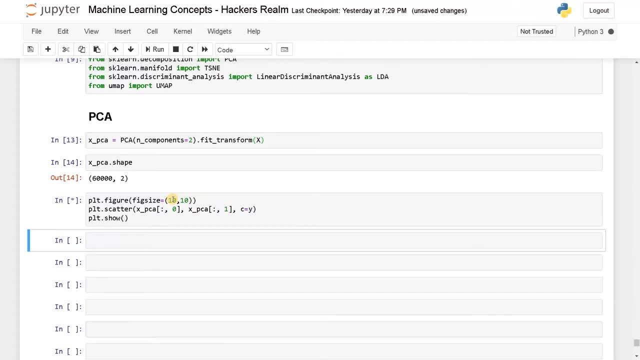 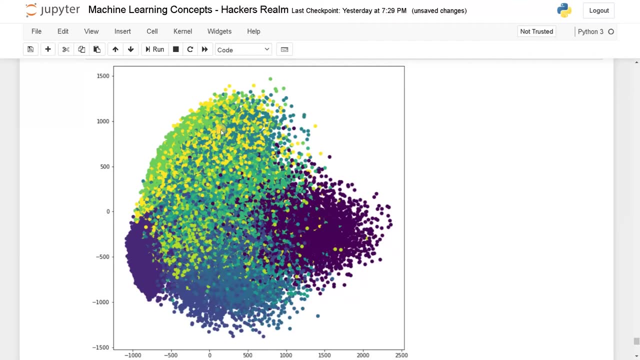 let's plot it now, And? okay, So this is somewhat bigger. I'll just reduce it to 10.. Okay, this is the whole data And, as you can able to see, it is like completely overlapping. Each color represents a particular digit, So this green represents one digit and this yellow. 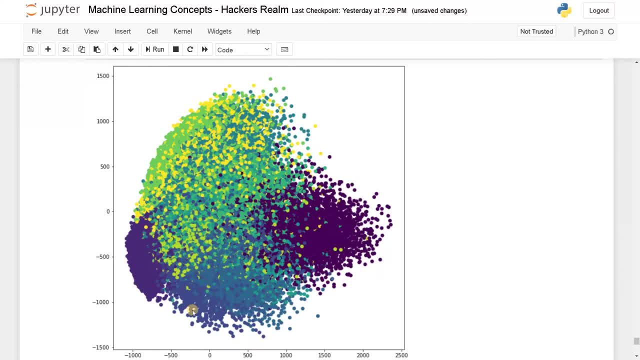 represents another digit And this violet and blue represents, like, each digit. But in the 2D representation we can clearly see most of the digits are overlapping and some of the digits are grouped together, like here, here in this violet and here this is: 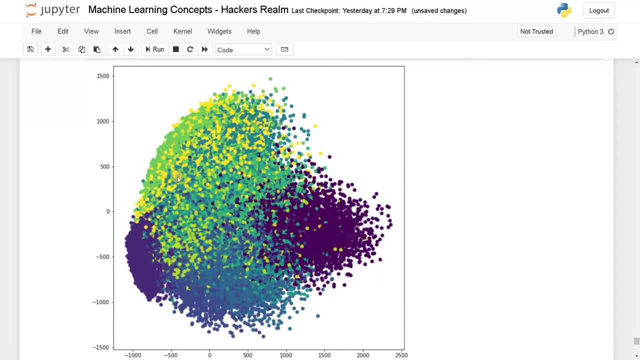 like dark violet And here this light green. everything is like grouped together, And even this yellow is also like grouped together. So this is how the feature reduction works. So if you have large amount of data, you can able to use these techniques in order to reduce. 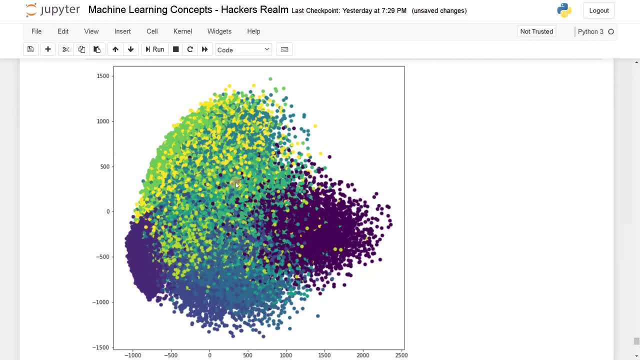 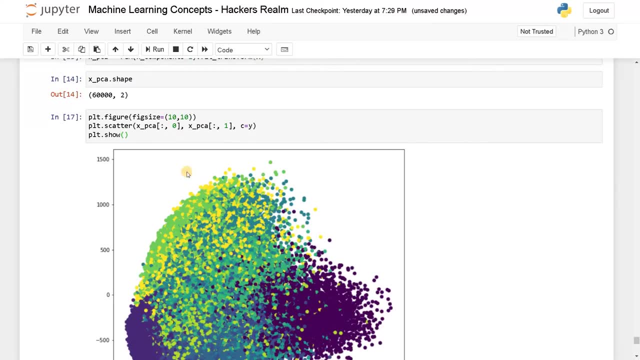 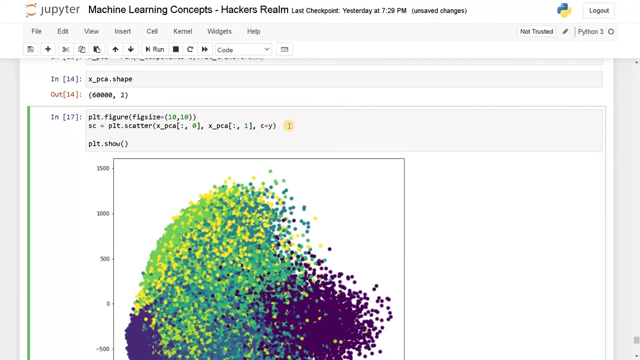 the number of dimensions. So this is a very helpful tool for training And this can also be used for visualization. So if you want to add legends, like if you want to label these colors, you can add like this: as equals. I'm just going to store this scatterplot and add this line, So I'm just 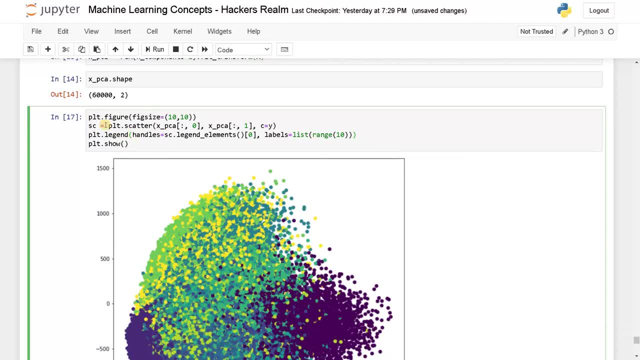 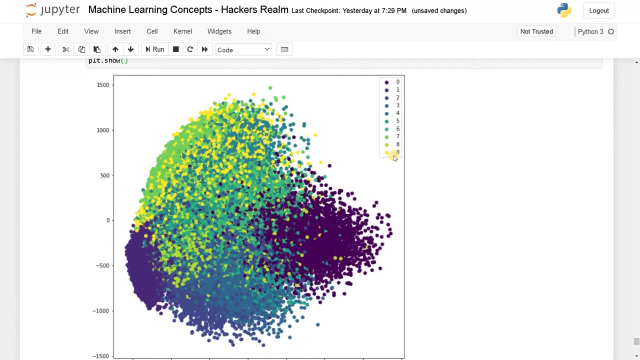 adding legends If you are using some kind of for loop and plotting the scatterplot means that will be different. So here I'm just creating a list of labels that is zero to nine, And uh, let's run this. Now you can able to see the colors. So each color color spawns to a digit. 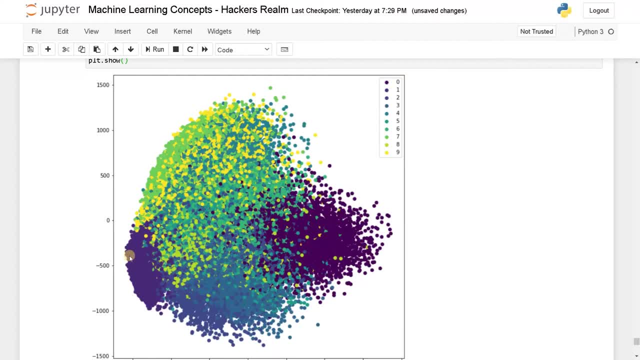 So here you can able to see I think this is zero and this is a one. I can't clearly differentiate between the color, because most of them are like somewhat similar. This eight and nine are all uh, uh club together. Uh, because you can obviously see eight also have. 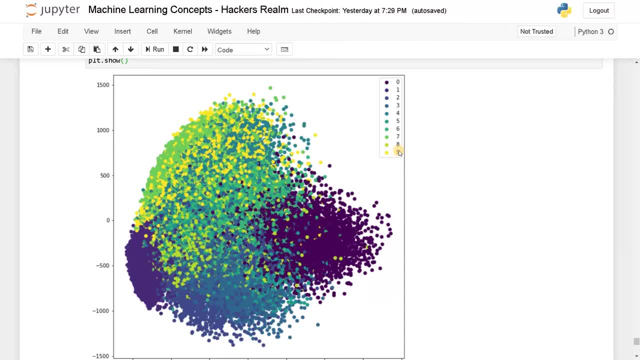 uh, a circle like a pattern. and nine also have the circle like pattern. And, uh, here six also will be having some kind of pattern. That's why these three are like overlapping to each other, and three, two are all, uh, overlapping here. So this is how the visualization 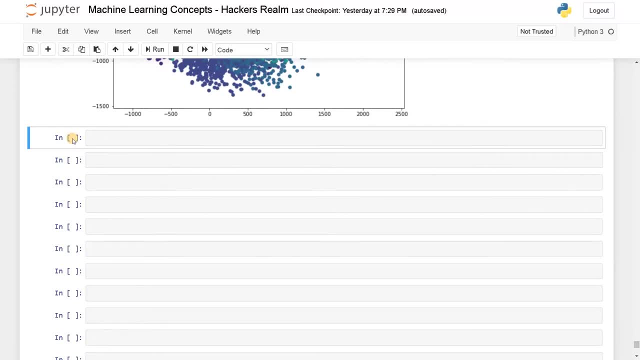 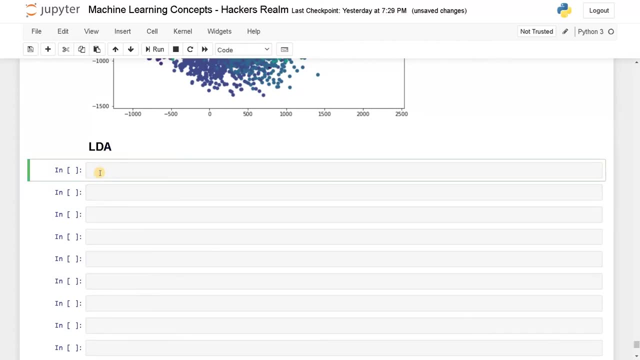 works. Now let's go for the next one. I'm going to go for LDA. So for LDA, we can do like this. So for LDA, we can do like this. uh, LDA equals LDA of similarly and components. It will be. 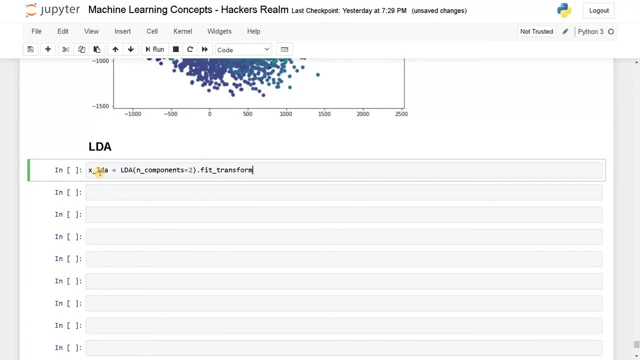 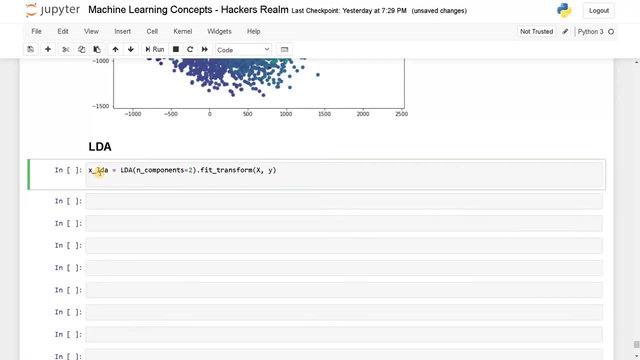 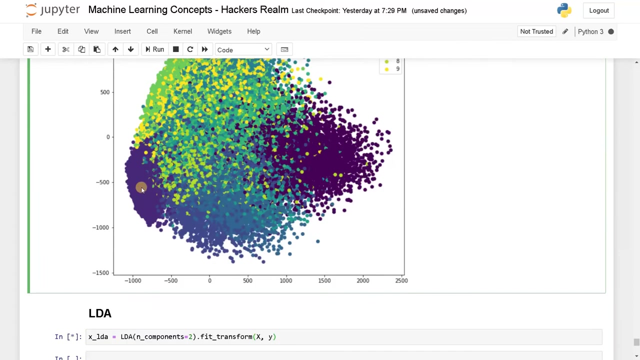 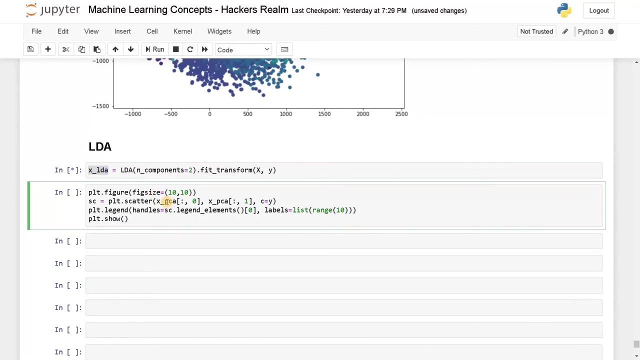 two. and for LDA we have to pass the output result, that is, the labels. So this will be X and Y and let's run this, And after that we will just do the same plotting here. instead of XPCA We'll be just using, uh, XLDA, okay, I think. uh, we have to wait for some time now. Yeah. 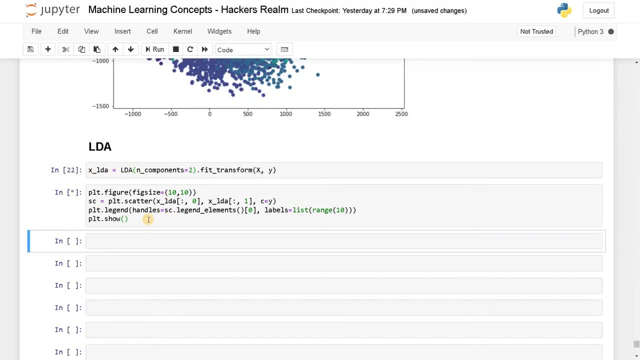 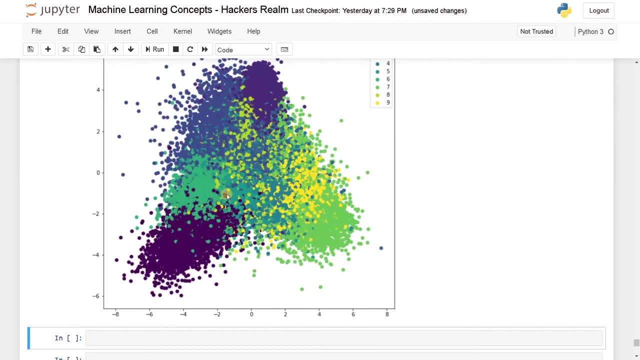 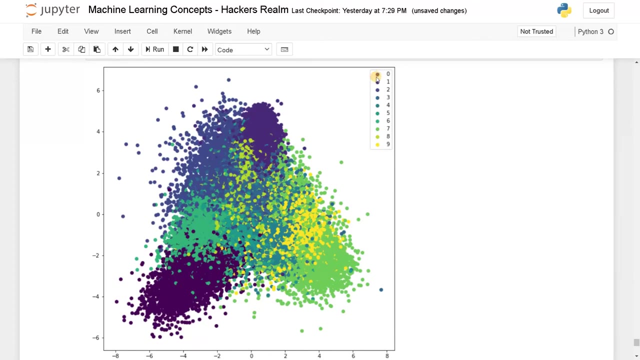 it's completed. Let's run this Now. again, you can see this LDA is producing some kind of a different results, but still, uh, some kind of overlapping you can clearly see and the grouping is also good. So here, uh, you can see eight and nine actually like close to each other, And if you also 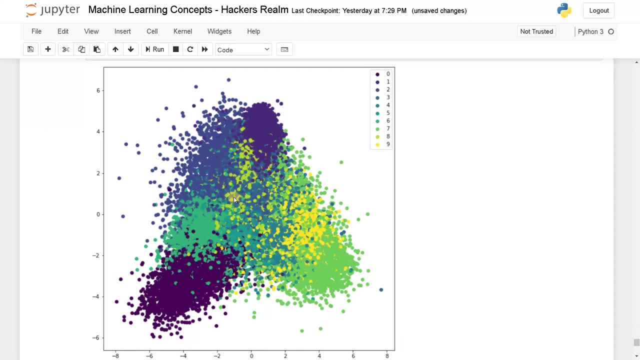 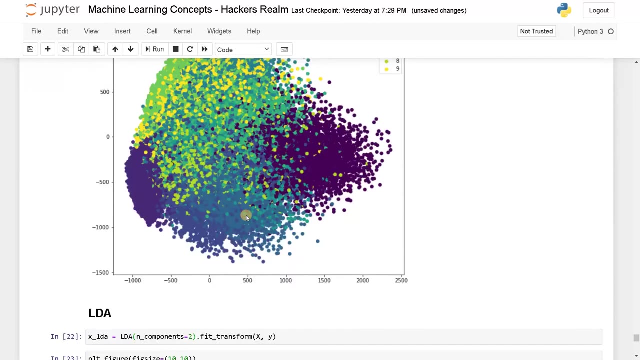 have like six also is uh near to eight. So and uh, these digits like zero and one is completely opposite, I guess, And two is in between. three is uh somewhere in behind because the colors are overlapping, but at least, uh, compared to this, this has like 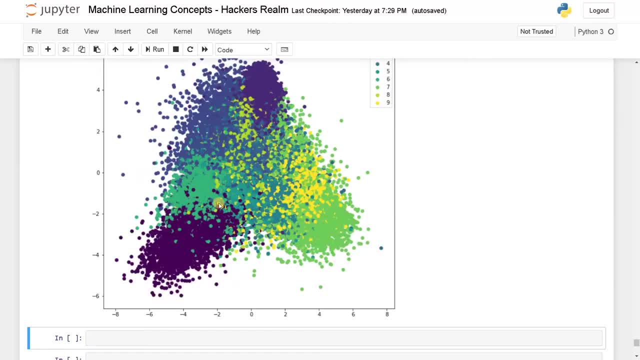 uh, uh, less number of overlapping. So, uh, I think it's still good. I think it's still good. So here, uh, you can see eight and nine actually close to each other, And if you also have some kind of overlapping, so this is somewhat better than PCA. Now let's go for. 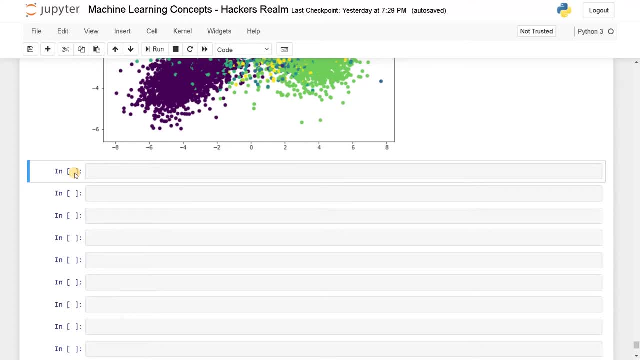 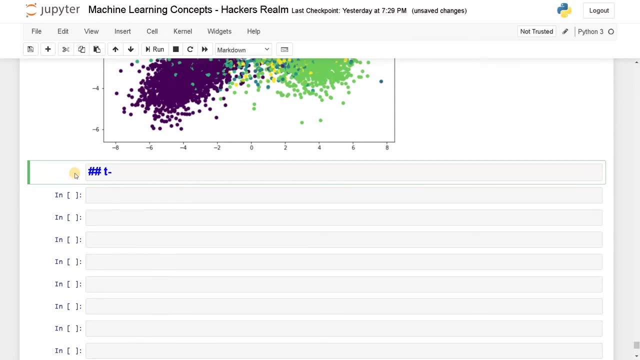 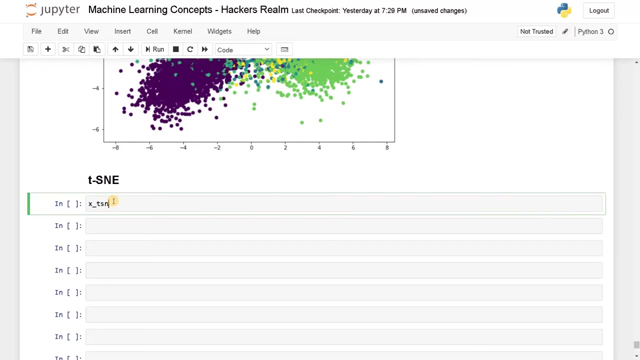 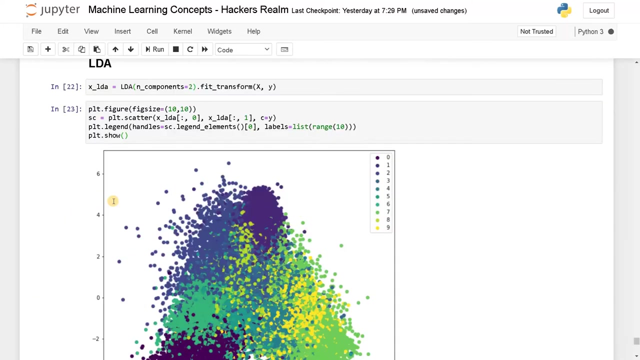 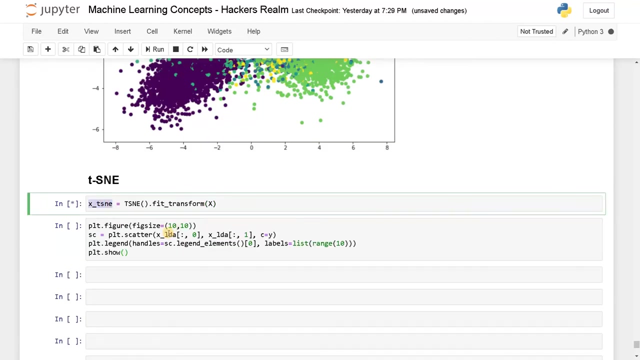 the next one, That is, uh, T S N E, T S N E. Okay, For this I'm going to use T S N? E equals T S N E of dot 50. Okay, Okay, So I'm going to run this. Let's copy this and paste it here Again. replace the variables. 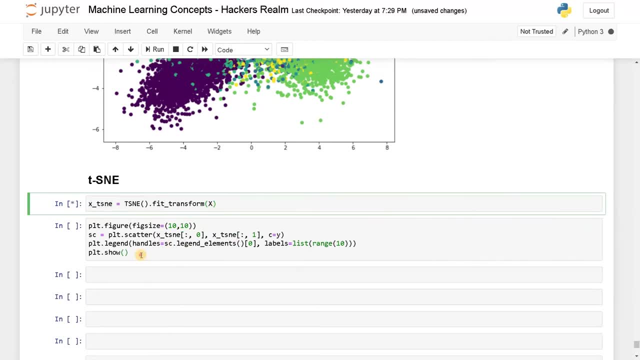 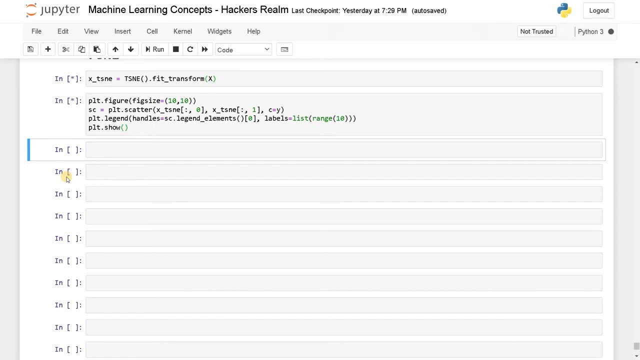 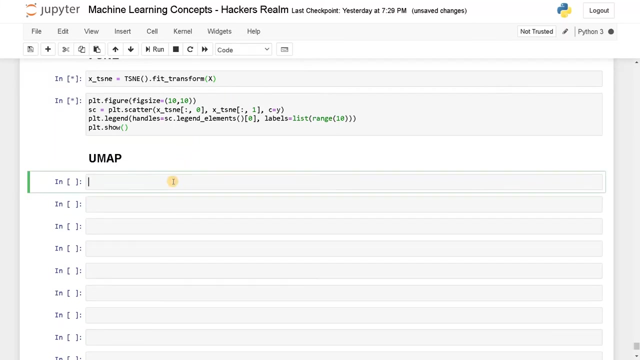 Okay, That's pretty much done. Let's also run this. So this is taking some time. in the meantime, create the syntax for you map also. so you map and for you map. just say x underscore you map equals you map of here we have to specify some parameters, so first it will be. 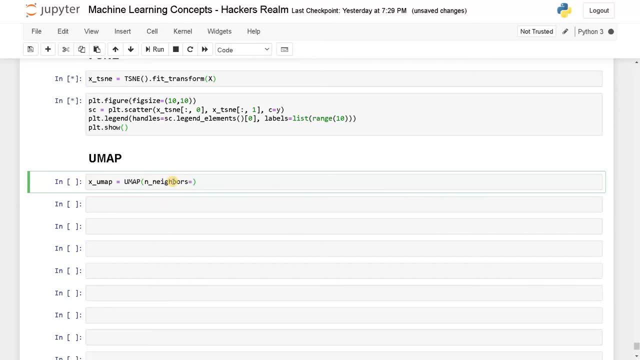 n neighbors, I will just say 10. so this is just for the grouping, and minimum distance equals 0.1. you can also go with the default parameters, so that is not a problem. metric equals correlation and now dot fit transform of x. So this will be done, and after that again we have to use the same plotting, just replace this. 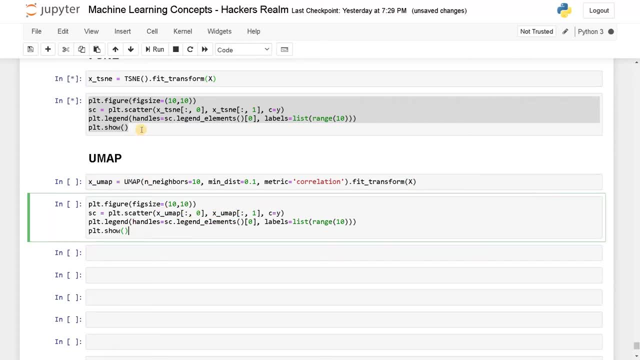 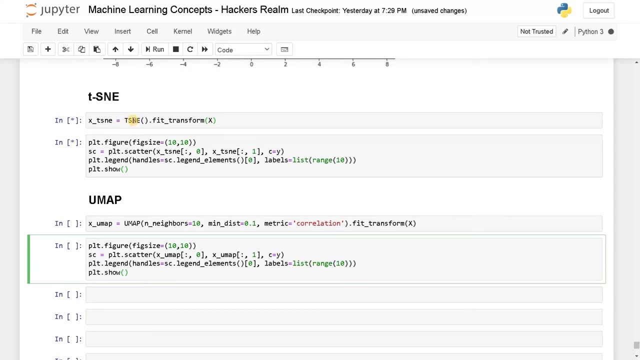 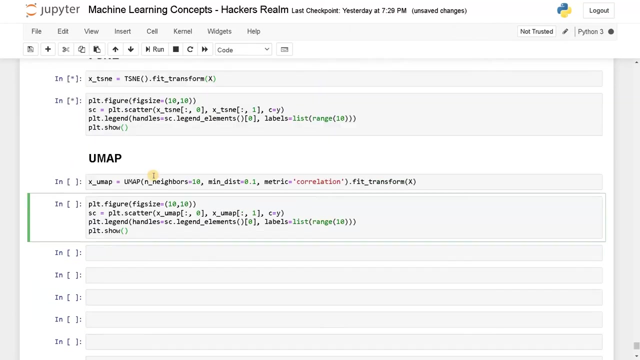 okay, that's pretty much done from our side, but we have to wait for TSN need to complete. the processing is taking so much long time compared to the above two modules. those two are like pretty quick for 60,000 samples. The processing has been done like instantly, but it's taking like more than a minute for. 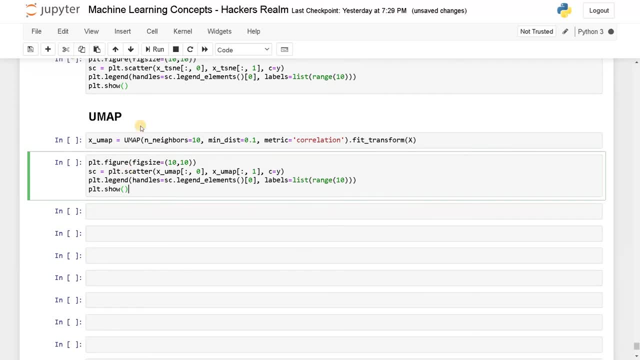 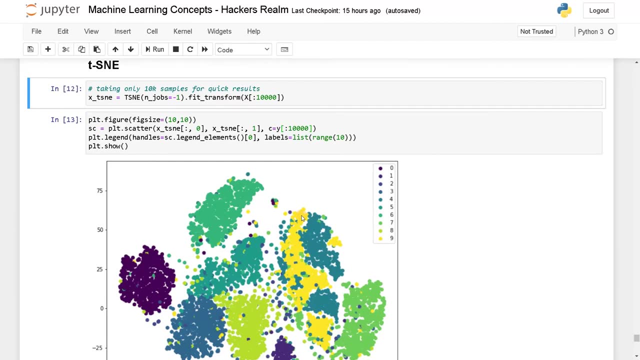 TSN need. its weight was some time and after that we will see how the results are going to be. so I just ran this TSN need for over an hour but it didn't give us a result. so I just tweaked few things. so I just used n jobs equals minus one to utilize all the course. 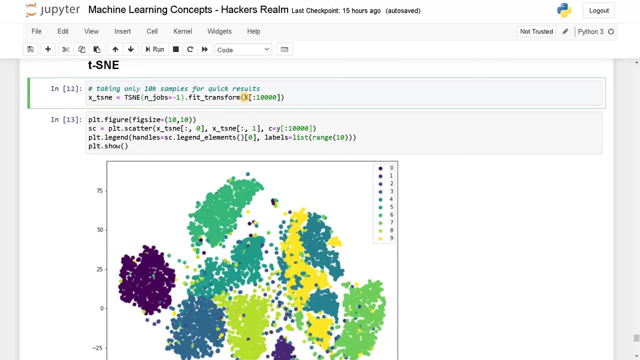 in my CPU And I also Felt Out like few samples, like I am taking the first 10k samples for quicker results. if you use all the 60k samples means it's taking more than an hour but still it's not giving. 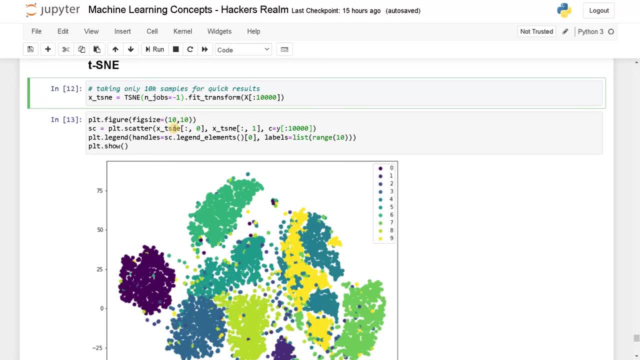 us the result. So for TSN need, if you want to utilize means, you can go for CUDA ML, because that utilizes GPU and can give you the results in like three seconds. so that is comparatively better than this. So this is pretty easy approach. Now let's explore the results. 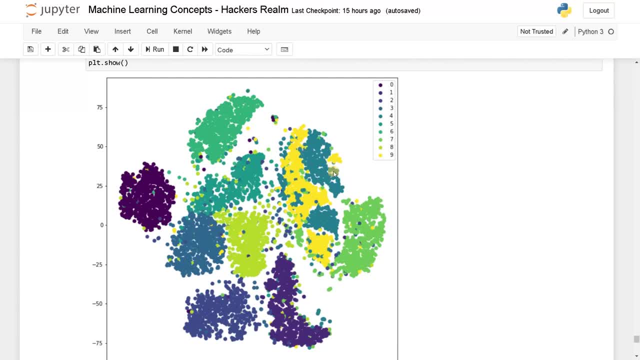 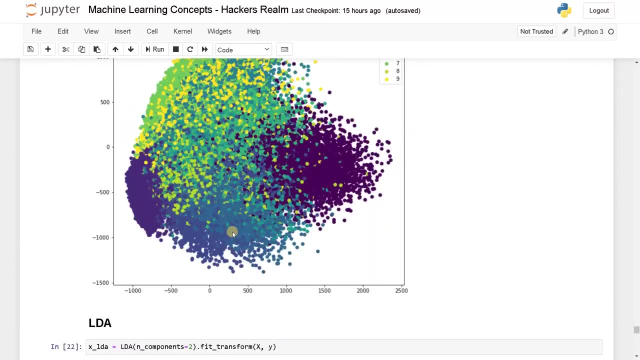 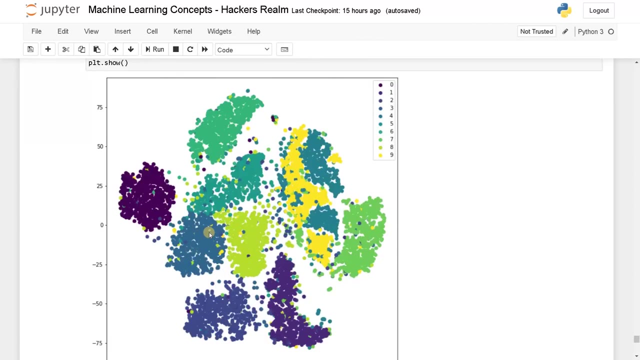 Here you can see a clear difference of clusters grouping with each other. all the attributes are like a group with each other and there is less overlapping compared to the previous two, that is, PCA and LDA. So the results are much clear and you can just use this two dimensional data for any 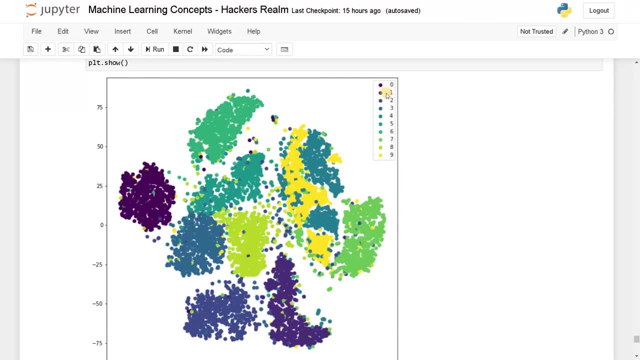 of the machine learning algorithms to classify the handwritten digits with less overlapping. As you can able to see, The results are much clearer and you can just use this two dimensional data for any of the machine learning algorithms to classify that handwritten digits with less overlapping. 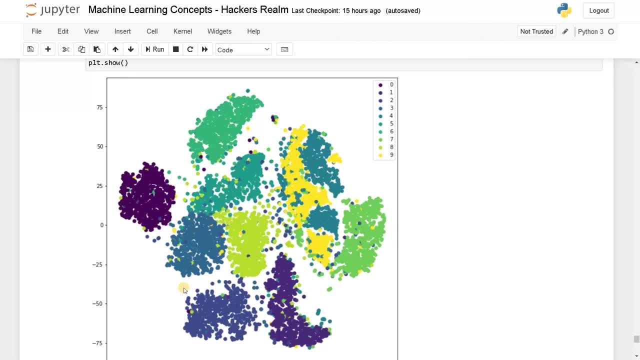 As you can able to see, here I have this one, which was a little bit overlapped, but now I have double-day data. see, you can clearly draw some decision boundary based on this, like two dimension. if you increase dimension a little means that will also give you a better results compared to this, but this is